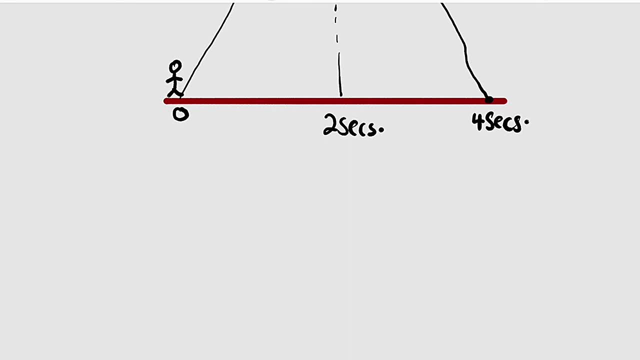 zero seconds. So let's form it. You know the general form. if you have a quadratic function as AX squared plus BX plus C, The vertex form will be Y equal to AX minus HO squared then plus K, where H and K here. 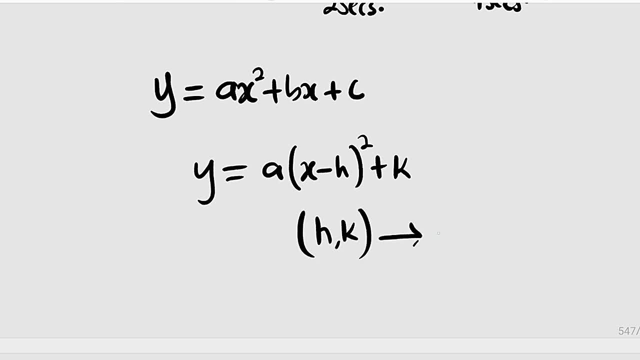 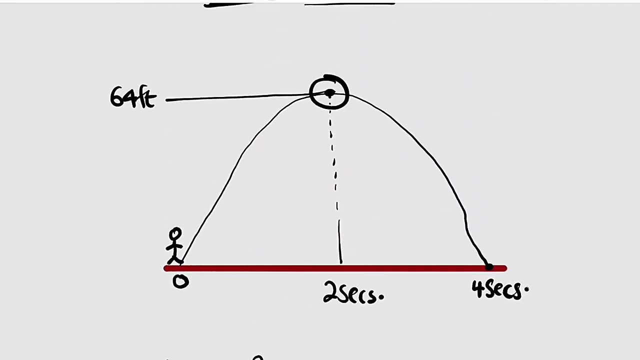 is a point which is the vertex, That is the maximum it can attain, right, That is this point. So at that point the height is 64 feet and the time is two seconds. Let us assume that the height is 64 feet, So we can substitute it there, But we are going to write the function. 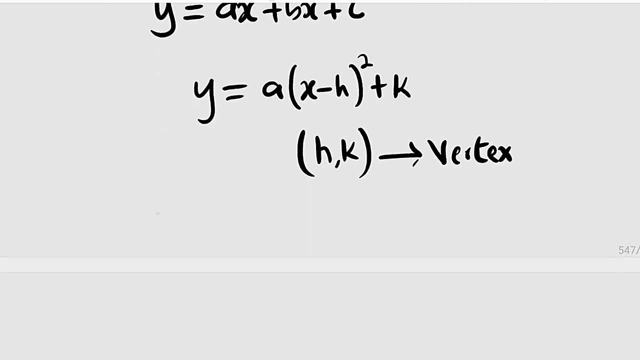 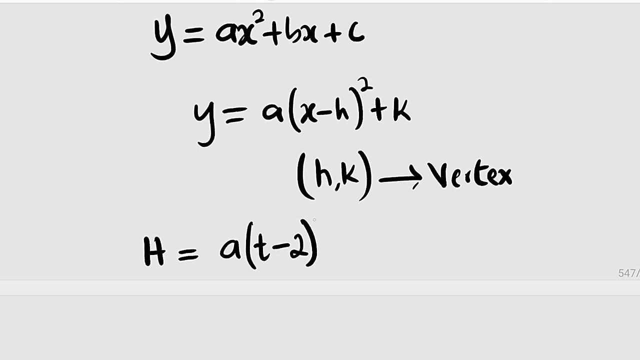 in terms of height and time, right. So H instead of Y, which is the height, is now equal to A. In the parenthesis, we have T instead of X minus H, which is what? Two seconds, We write, two here, We square all, Then we add the maximum height, which is 64.. So all we need to find. 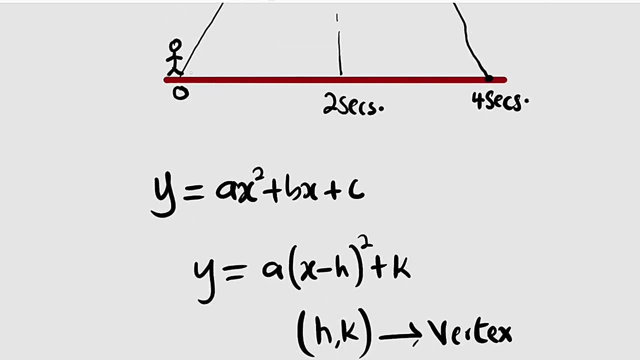 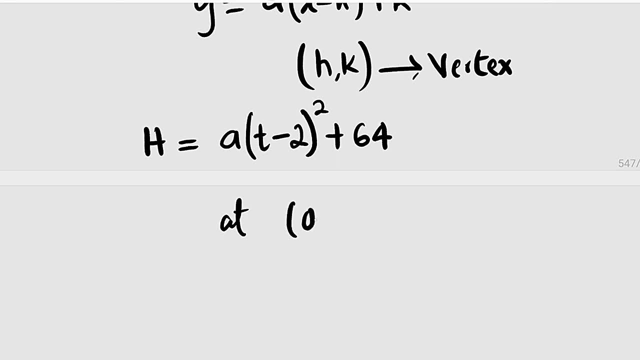 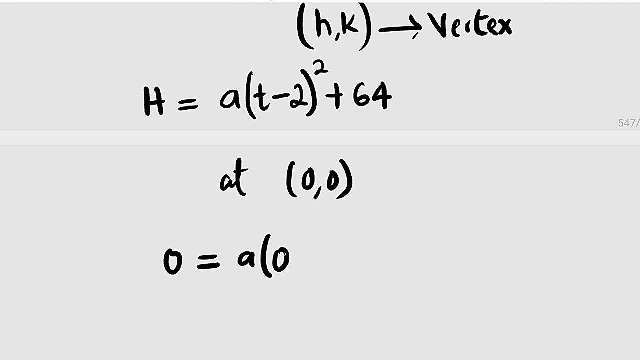 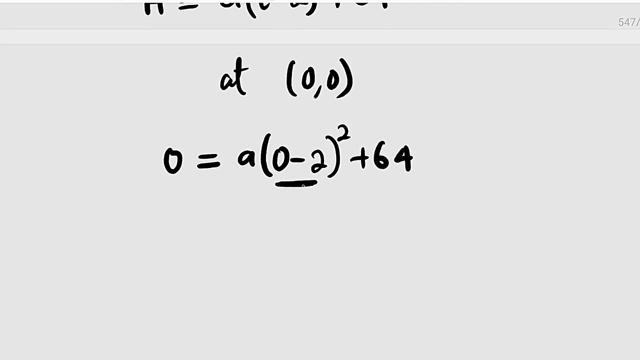 is the value of A And we can pick any point. Let us pick the origin, where bus time and height are equal to zero. So at zero zero we have H to be zero. equal to A Time is also zero. Square them plus 64. We have zero minus two, which. 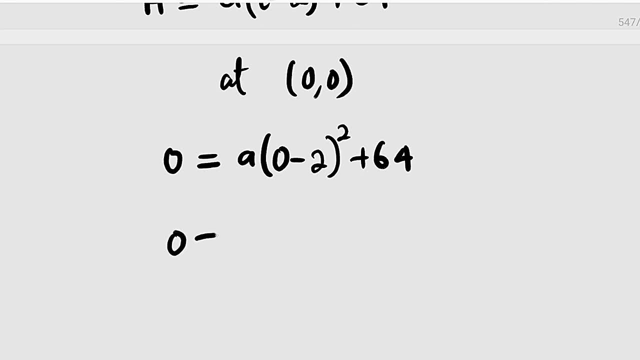 is negative two. If you square that, you get four. So this is zero equal to four A plus 64. If you take 64 to the other side, it becomes negative. We have four A equal to negative 64. You divide both sides by four. A will now be equal to negative 64 divided by four. 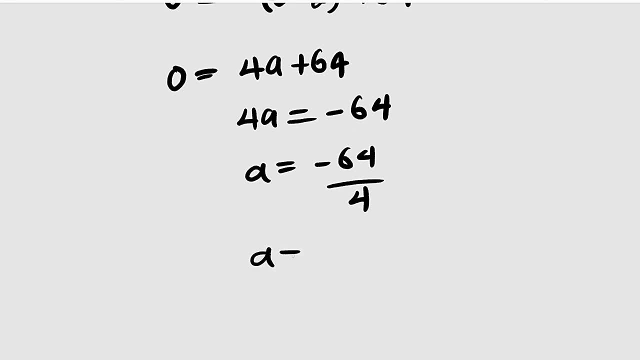 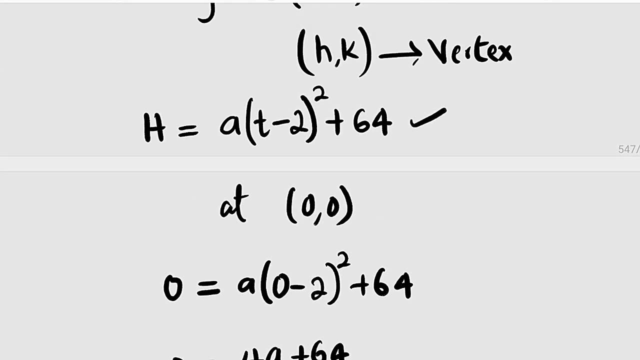 And negative 64 divided by four is negative 16.. Therefore, A is equal to negative 16.. So now let us plug in A into this vertex form of our parabola. So H, which is a function of time, is equal to A, which is negative 16.. 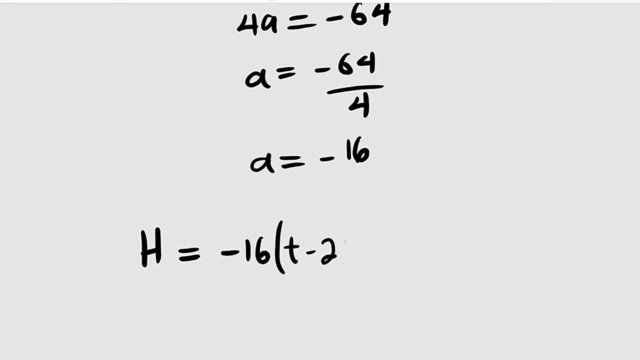 And H, which is a function of time, is equal to negative 16.. So minus H, which is negative, 16, multiplied by T minus two, all squared then plus 64. So this is the relationship between the height and the time, And if you expand this you are going to obtain that. 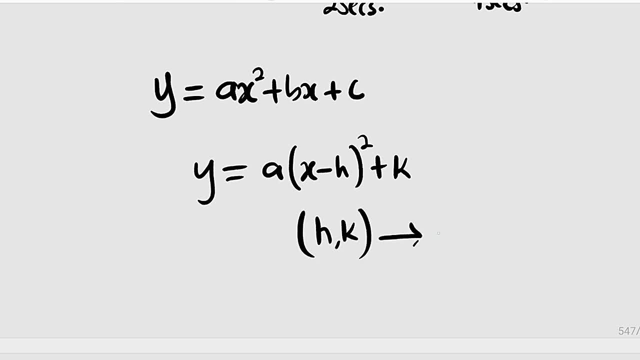 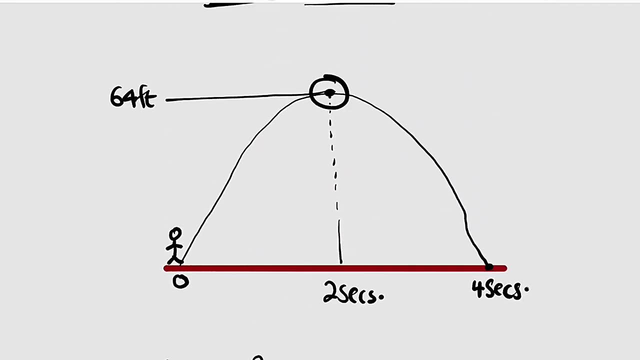 is a point which is the vertex, That is the maximum it can attain, right, That is this point. So at that point, the height is 64 feet and the time is two seconds. Let us assume that we have substituted there, But we are going to write the function in terms of height. 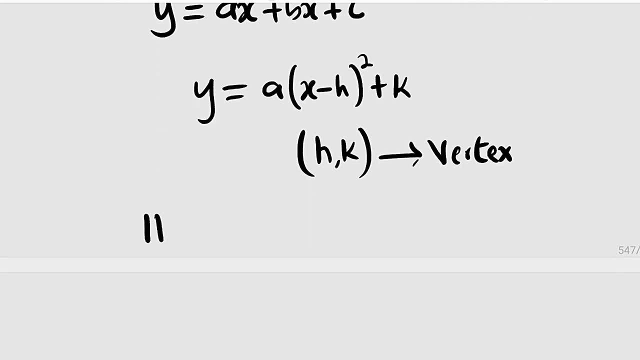 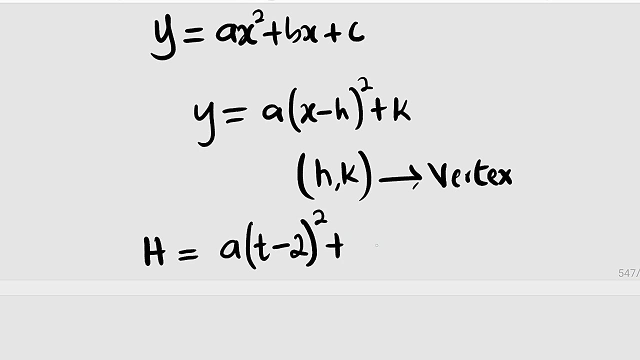 and time right. So H instead of Y, which is the height, is now equal to A. In the parentheses we have T instead of X minus H, which is what? Two seconds We write two here, We square all, then we add the maximum height, which is 64.. So all we need to find is the value. 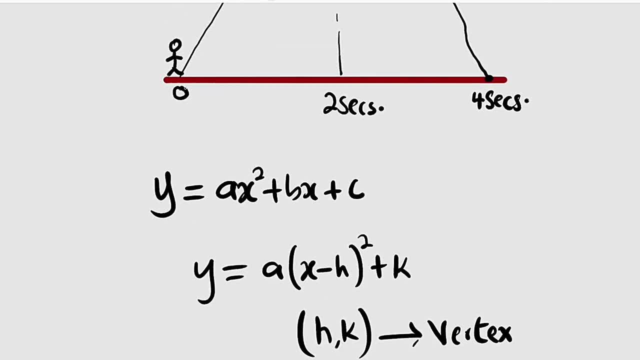 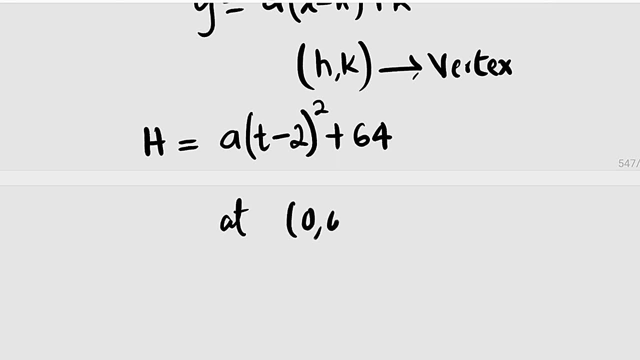 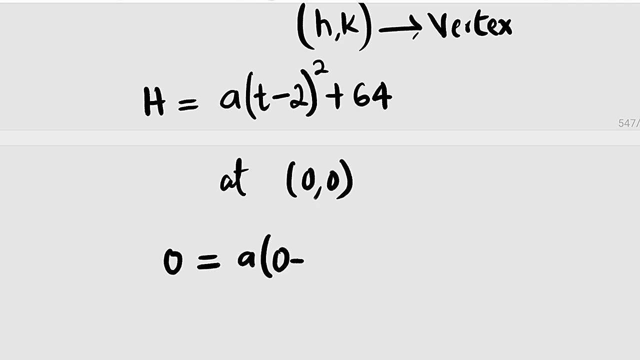 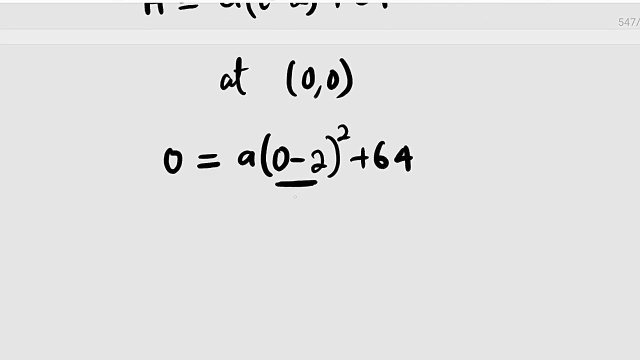 of A and we can pick any point. Let us pick the origin, where bus time and height are equal to zero. so at zero zero we have h to be zero. equal to a time is also zero. squared then plus 64, we have zero minus two, which is negative two. 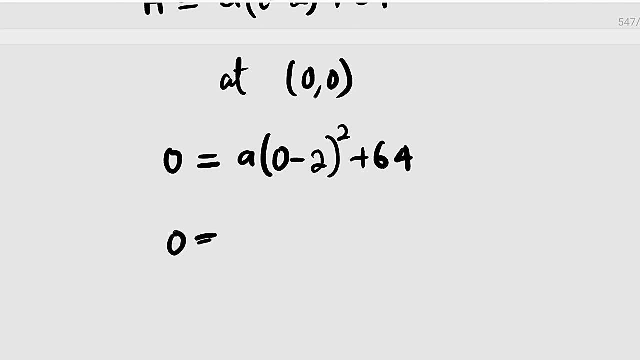 if you square that, you get four. so this is zero equal to four, a plus 64. take 64 to the other side. it becomes negative. we have four a equal to negative 64. you divide bus size by four: a will now be equal to negative 64 divided by four. and negative 64 divided by four is negative 16. 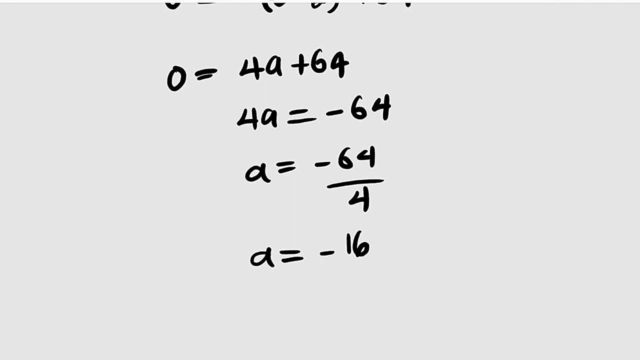 therefore a is equal to negative 16. so now let us plug in a into this vertex form of our parabola. so h, which is a function of time, is equal to a, which is negative 16, multiplied by t minus two. all squared, then plus 64. so this is the relationship between the height. 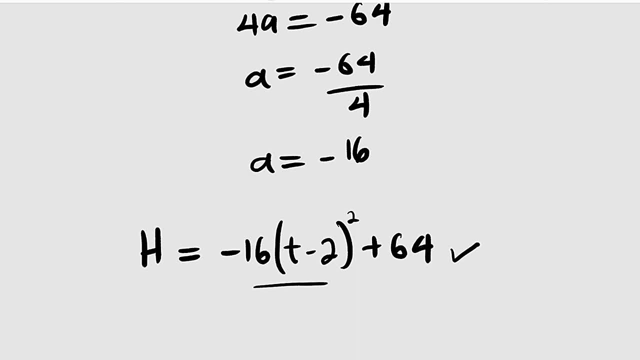 and the time, and if you expand this, you are going to obtain that quadratic equation which we have used to form this graph. let us do it as a bonus. h is now equal to negative 16. if you expand this first time squared, which is t squared minus two times the first time, times the second time will give us: 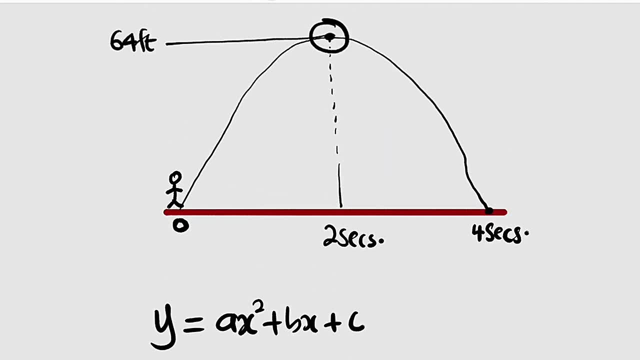 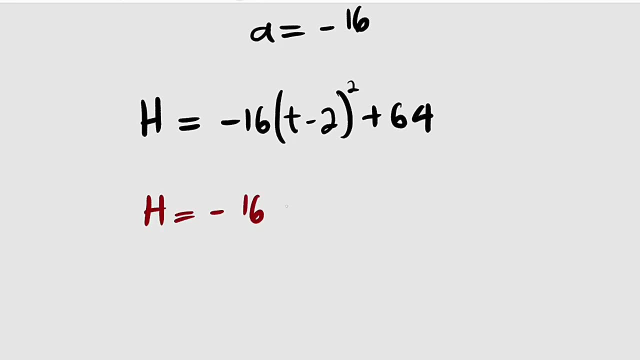 quadratic equation which we have used to form this graph. Let us do it as a bonus: H is now equal to negative 16.. If you expand this first times squared, which is T squared minus H. So now what we need to do is that we multiply the square root of X by two A. 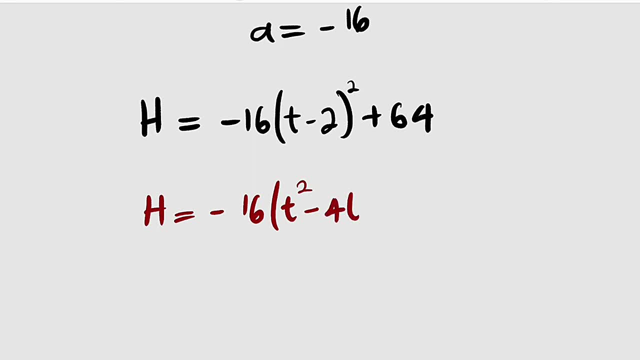 us 2 times the first time. times the second time will give us 4t negative. Then negative 2 squared will give us 4, then plus 64.. Let us expand the parenthesis: Negative 16 times t squared will give us negative 16t squared. 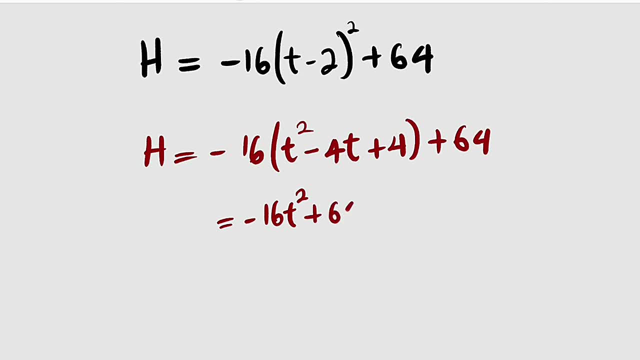 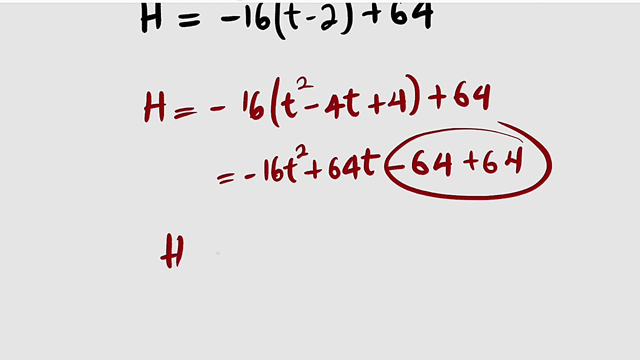 Negative, negative positive 16 times 4 is 64t. Negative positive is negative 16 times 4 is 64. Then we have our 64. This will give us 0, right? So therefore our function h is equal to negative 16t squared plus 64t. This is the quadratic. 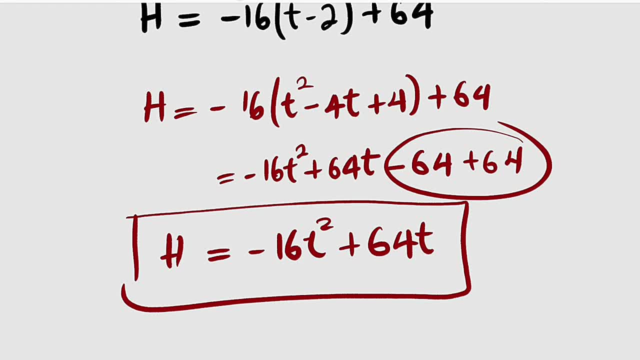 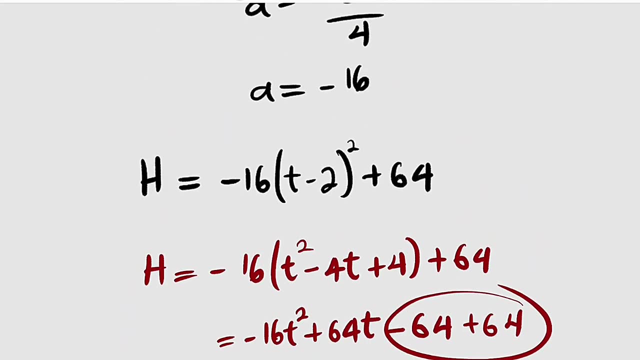 equation used to construct that graph, But this is not what we are looking for. We are looking for the time, O times- at which the ball reaches what? 48 feet, So, when h is equal to 48 is exactly what we are looking for, And I'm going to use the 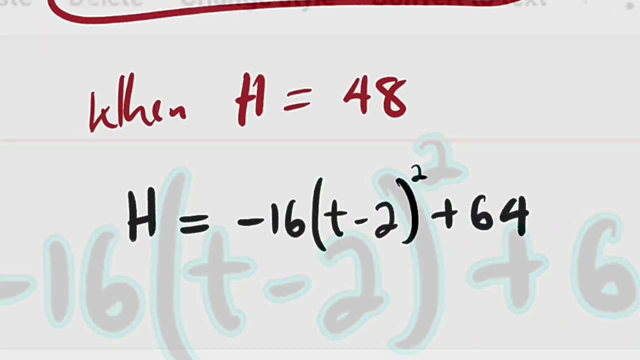 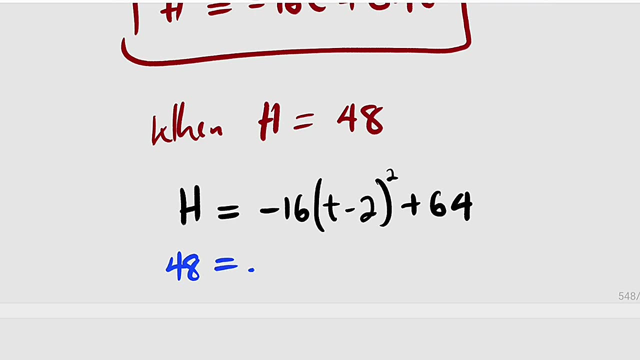 vertex form, which is very simple. Let me use this. So this is the vertex form of our quadratic equation, where h is now 48, equal to negative 16, multiplied by t minus 2, all squared plus 64.. Let us take this time to the left-hand side and take 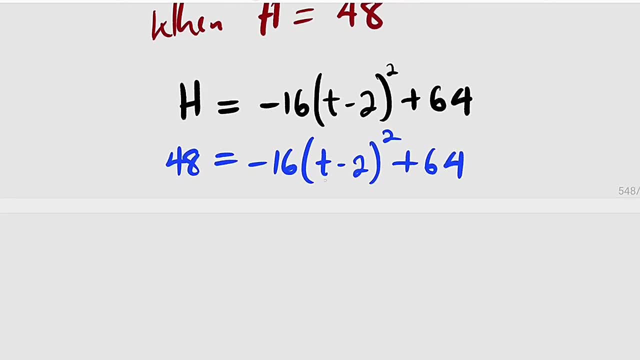 this one to the right-hand side. We're just going to switch them. As this time crosses the equality sign, it becomes positive. 16t minus 2 all squared. If this one crosses over, it becomes negative. So we have 64 minus 48.. And 64 minus 48 is 16.. 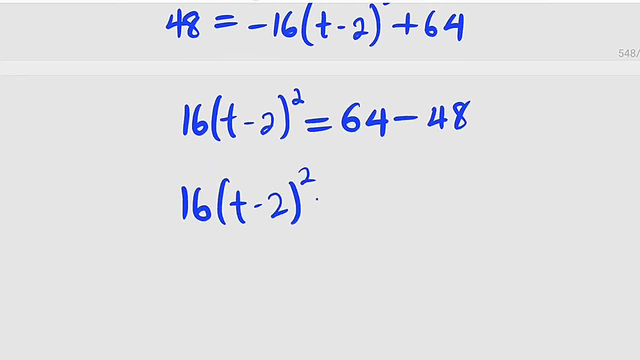 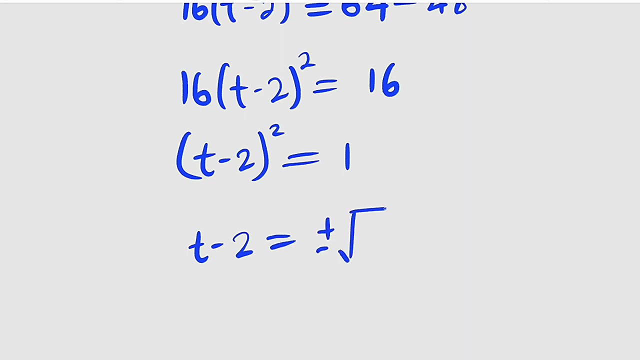 So we have 16t minus 2, all squared equal to 16.. Divide both sides by 16. You have t minus 2, all squared equal to 1.. Take the square root of both sides. You have t minus 2, equal to plus or minus the square. 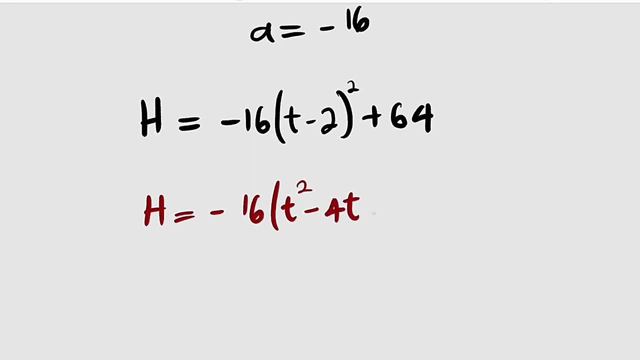 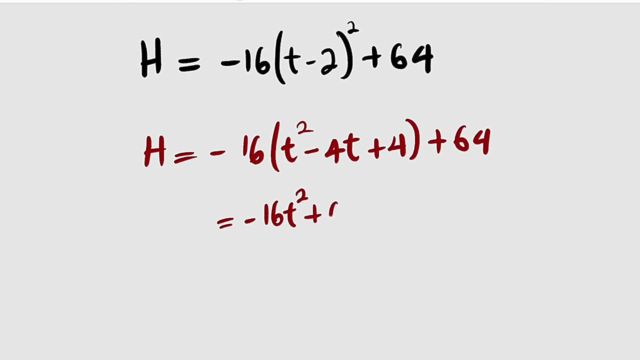 four t negative, then negative. two squared will give us four, then plus 64. let us expand the parentheses. negative 16 times t squared will give us negative 16 t squared. negative, negative, positive 16 times four is 64 t negative. positive is negative. 16 times four is 64, then we have our 64. this will give us zero. 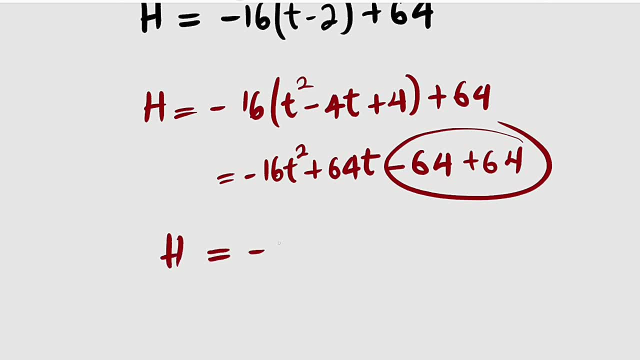 all right. so therefore our function h is equal to negative 16 t squared plus 64 t. this is the quadratic equation used to construct that graph. but this is not what we are looking for. we are looking for the time o times at which the ball reaches the75Ba decorating equation. just Rück 한� saflie. 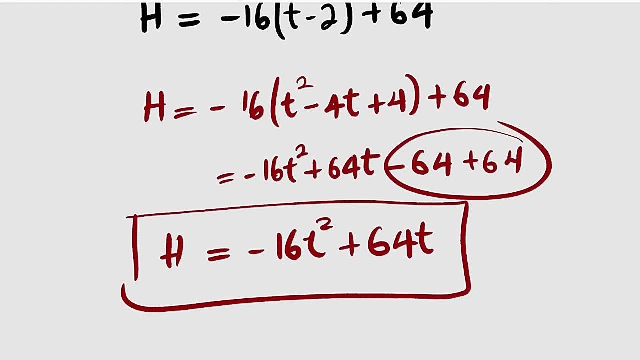 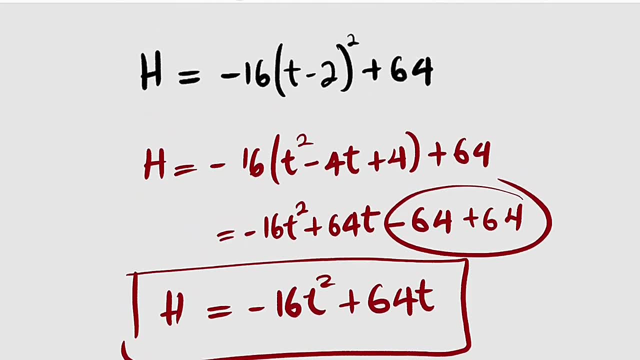 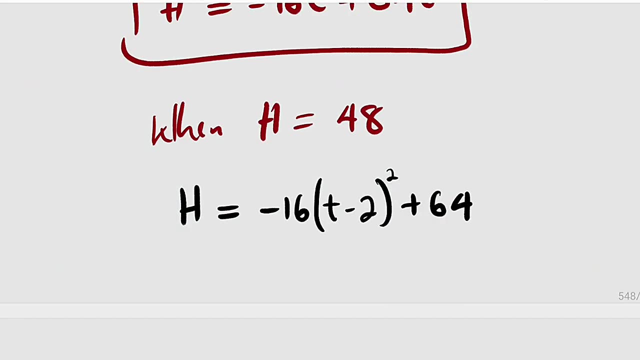 almos 60af. what 48 feet? so when h, when h is equal to 48, is exactly what we are looking for, and i'm going to use the vertex form, which is very simple. let me use this. so this is the vertex form of our quadratic. 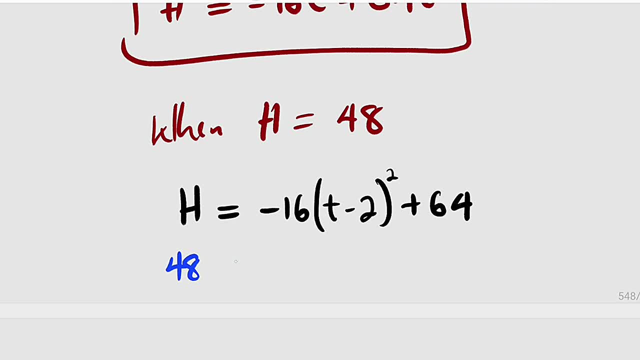 equation where h is now 48, equal to negative 16 multiplied by t minus 2, all squared plus 64. let us take this time to the left hand side and take this one to the right hand side. we're just going to switch them. as this time crosses the equality sign, it becomes positive. 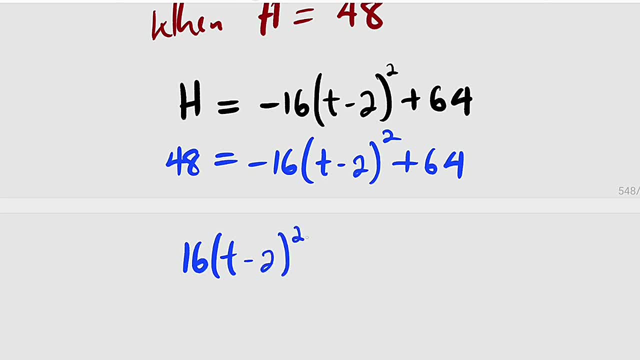 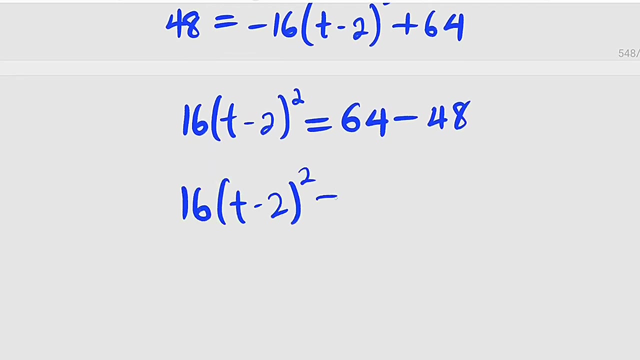 16. t minus 2, all squared. if this one crosses over, it becomes negative. so we have 64 minus 48, and 64 minus 48 is 16. so we have 16. t minus 2, all squared equal to 16. divide both sides by 16. you have t minus 2, all squared equal to 1. take the square root of both. 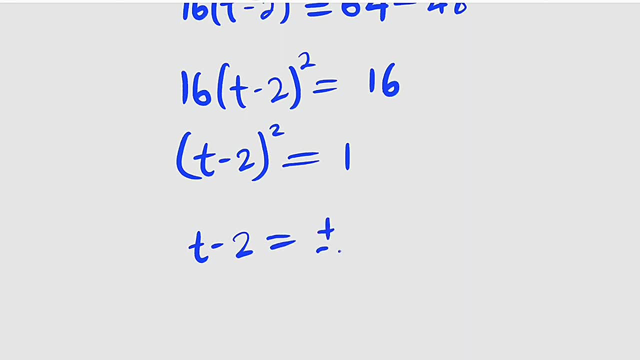 sides, you have t minus 2, equal to plus or minus the square root of 1, which is the same thing as 1. take negative 2 to the right hand side. t will now be equal to positive 2 plus or minus 1, because square root of 1 is 1. so, finally, the time that we are looking for is equal to either 2 plus 1.